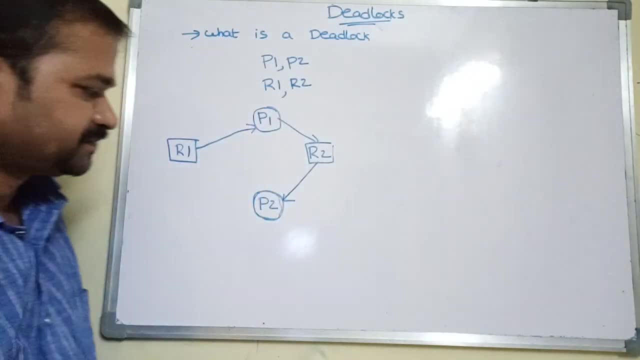 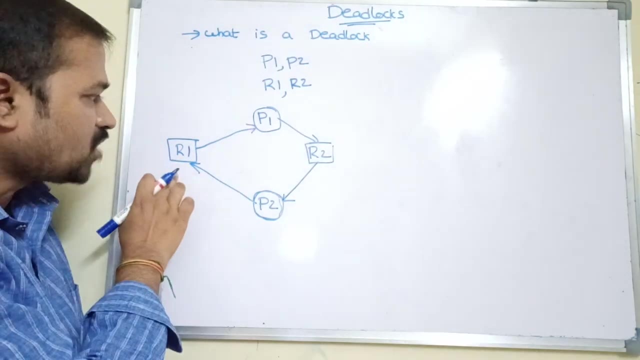 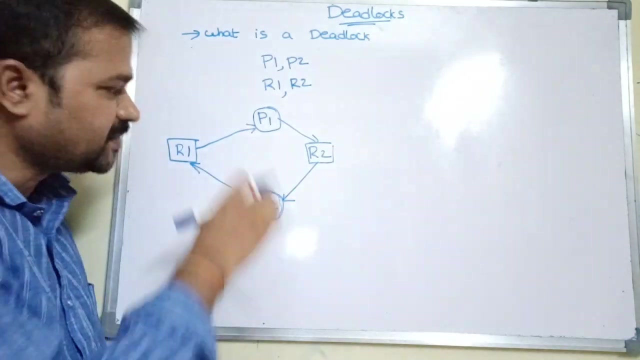 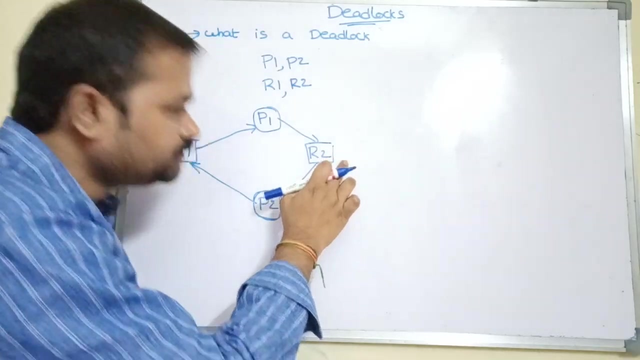 So operating system can't allocate R2 to P1.. Next, let us assume that P2 has put a request for resource R1. Here R1 is allocated to P1. So operating system can't allocate R1 to P2.. So here the situation is: P1 has acquired resource R1 and it is waiting for R2, but R2 is acquired by P2.. 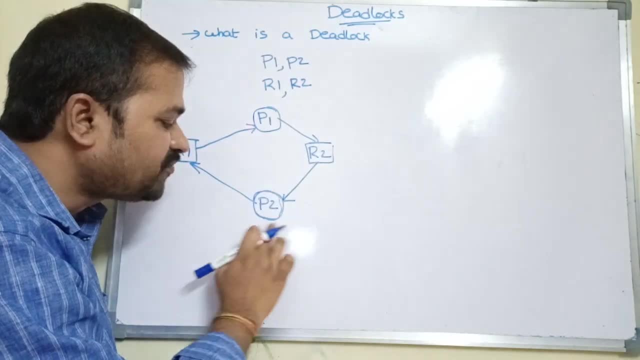 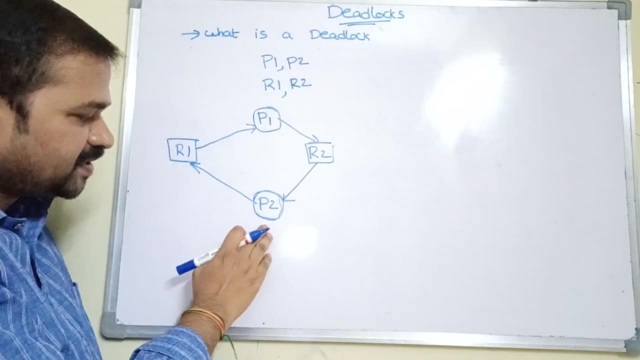 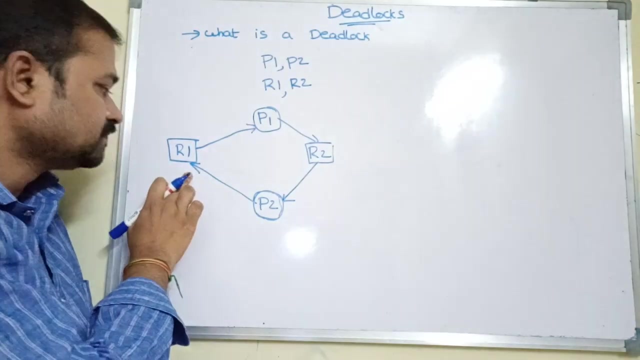 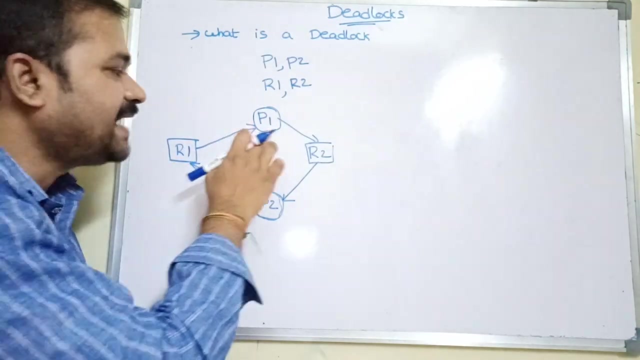 P2 can release R2 only after its completion. So P2 cannot release R2.. Next point: P2 has acquired resource R2 and is waiting for R1, but R1 is acquired by P1.. P1 cannot release R1 until and unless it has completed its execution. 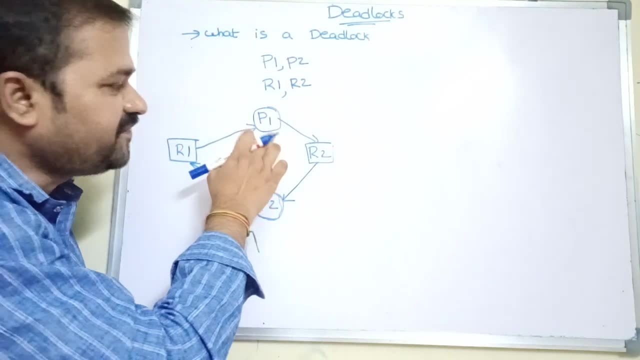 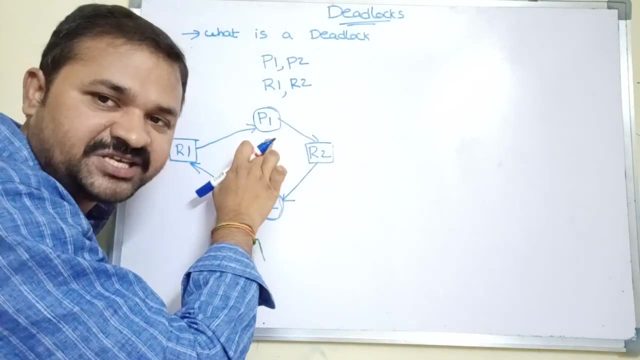 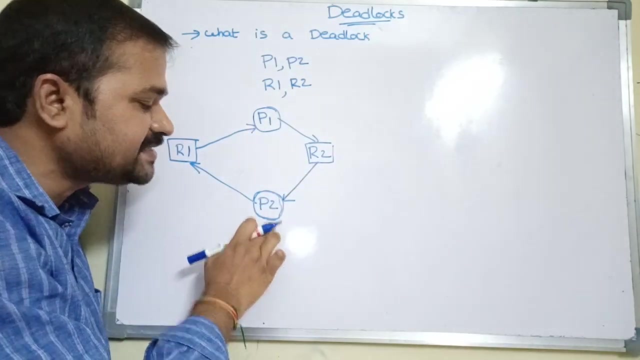 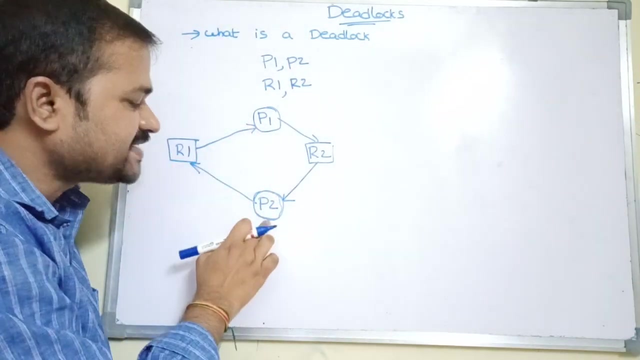 So here the point is: P1 cannot release the resource R1 until and unless P1 completed its execution. Likewise, P2 cannot release resource R2 until and unless it completed its execution. So P1 cannot release the R1, as well as P2 cannot release the R2.. 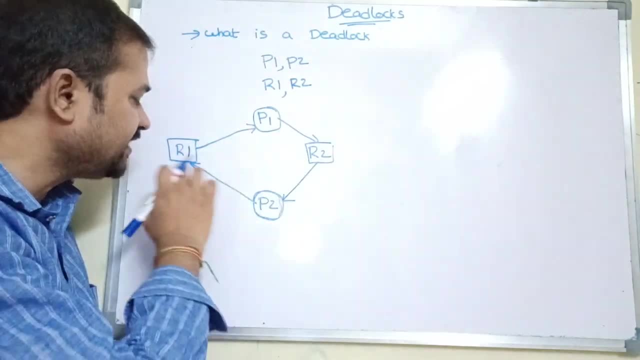 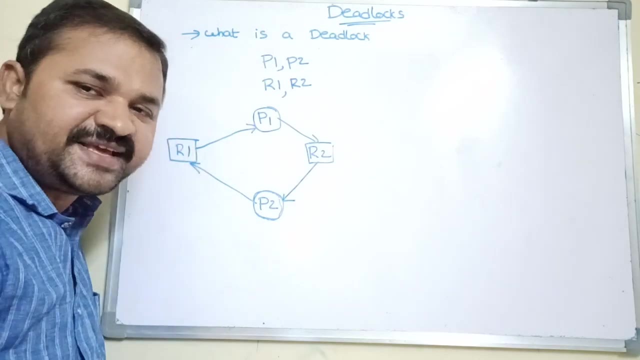 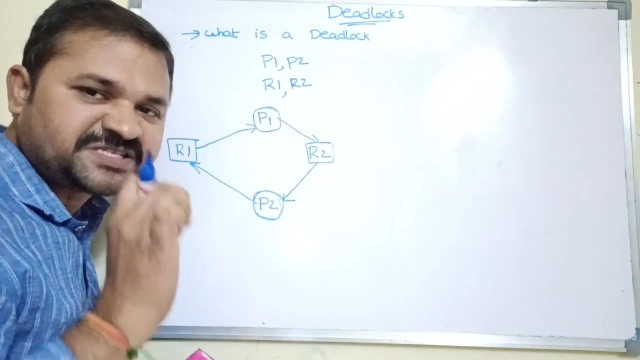 Why? because, in order to execute the process, P1 requires both these resources. Likewise, P2 requires both these resources. This situation is known as deadlock. Why? because in this situation, we can't execute P1 process as well as P2 process, So we can call this situation as a deadlock. 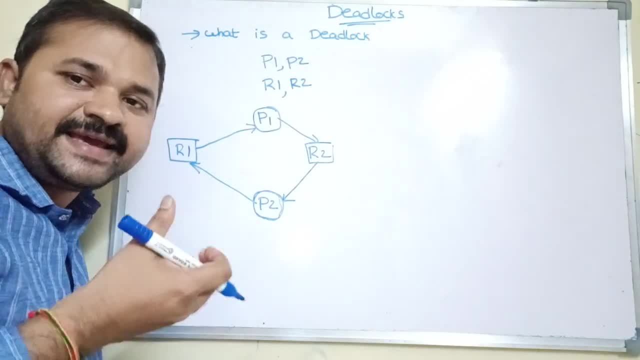 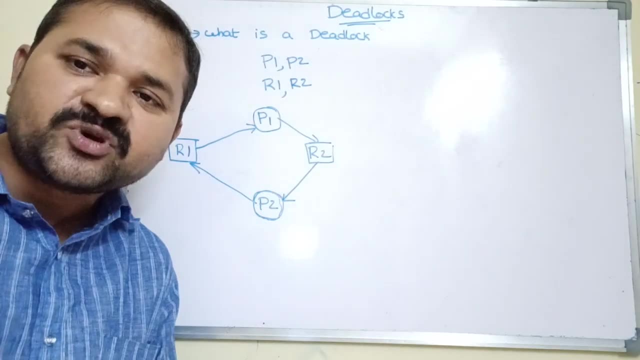 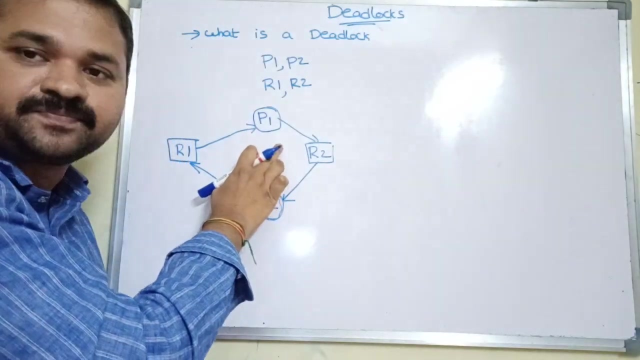 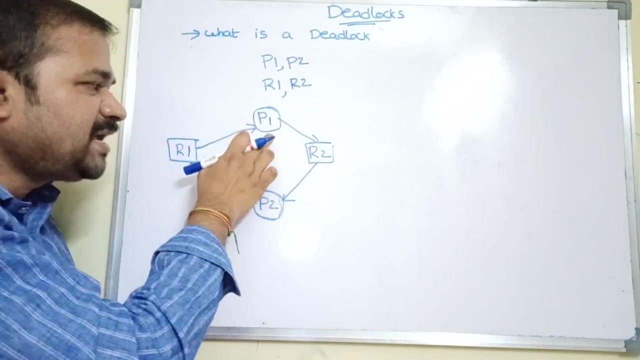 Now let's see the definition for a deadlock. A set of processes are set to be in deadlock If every process is holding some resources And is waiting for additional resources, But which are acquired by another process. If you take this example, P1 is holding R1.. 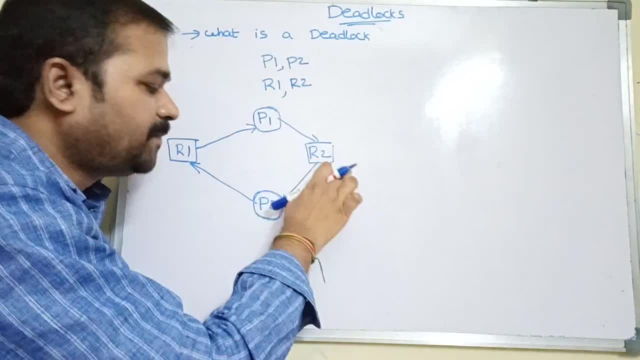 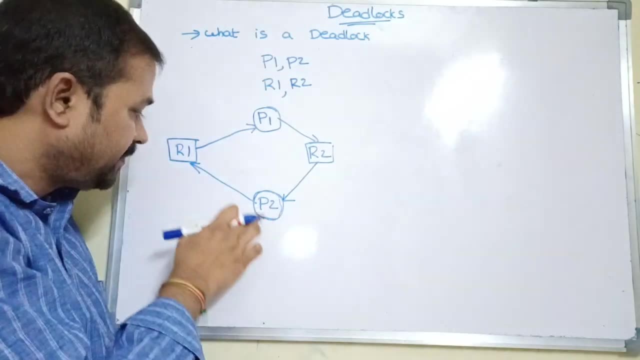 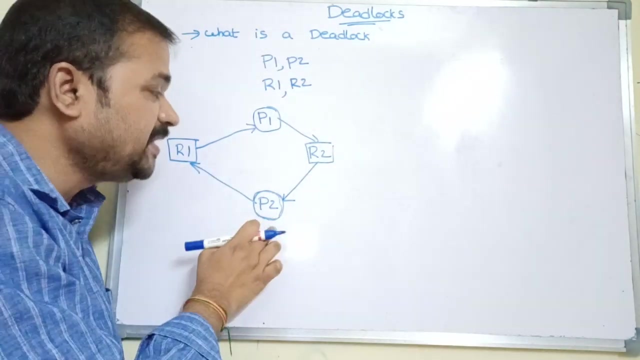 And it is waiting for R2.. But R2 is acquired by P2.. But P2 can't release R2.. Why? because P2 requires R1 also for its completion. Only after getting P1. R1, only P2 releases R2.. 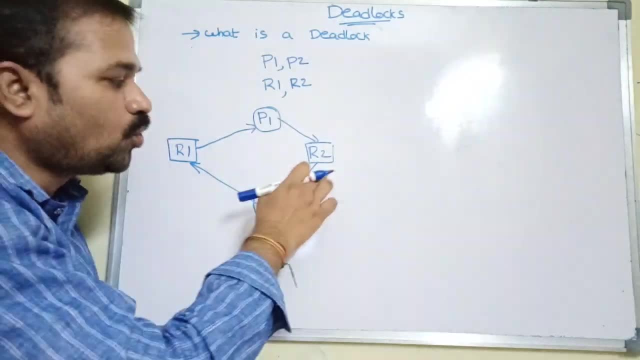 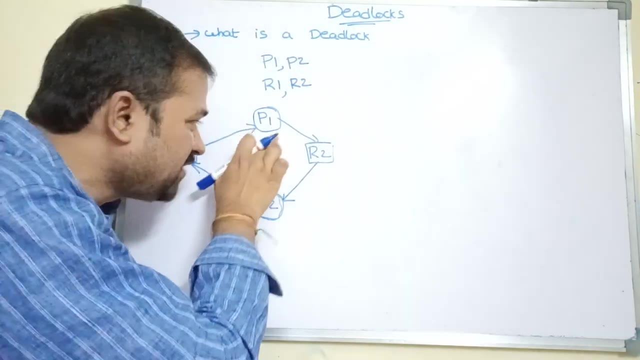 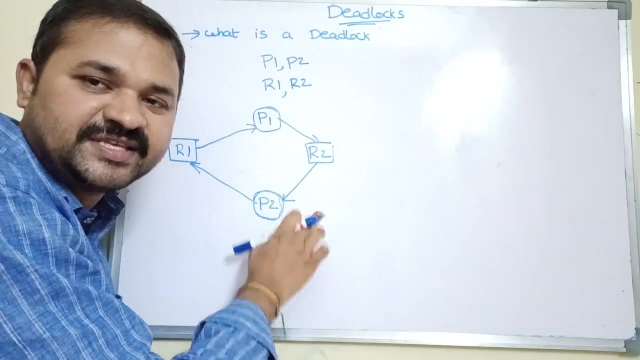 If you take about P2.. P2 is holding R2. And it is waiting for R1. But R1 is acquired by P1. But P1 can't release R1. Why? because it is waiting for R2 also. So this is the definition for a deadlock. 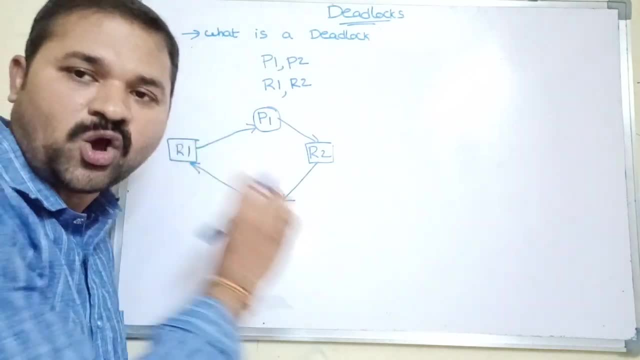 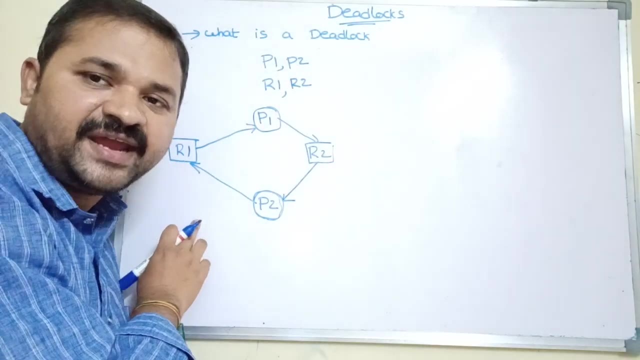 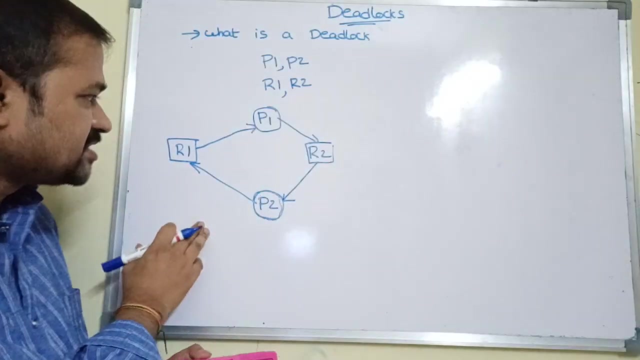 A set of processes are set to be in deadlock state If every process in the set is holding some resources And waiting for additional resources, But which are released by other process. Here, what are the set of processes? We have two processes, P1 and P2.. So this is the definition for a deadlock. 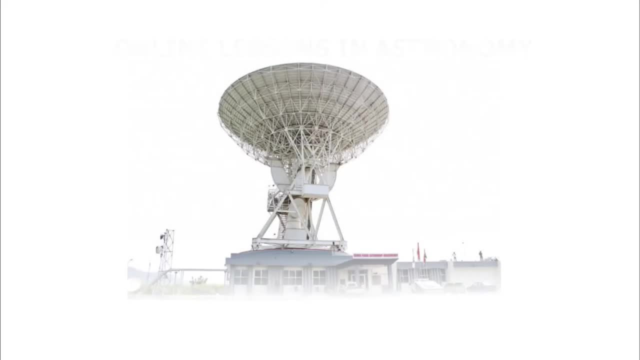 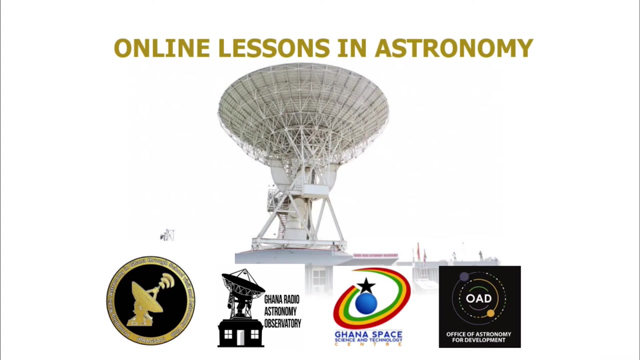 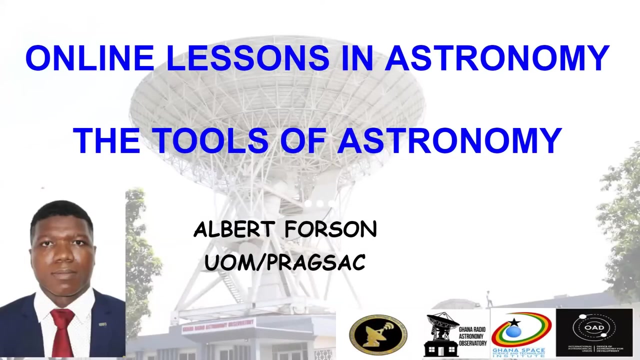 Hello everyone. I am Albert Fawcett. I welcome you to Online Lessons in Astronomy. The topic is the tools of astronomy. In our previous lessons we had lessons on the solar systems, our place in the universe, and also on electromagnetic spectra. Today, 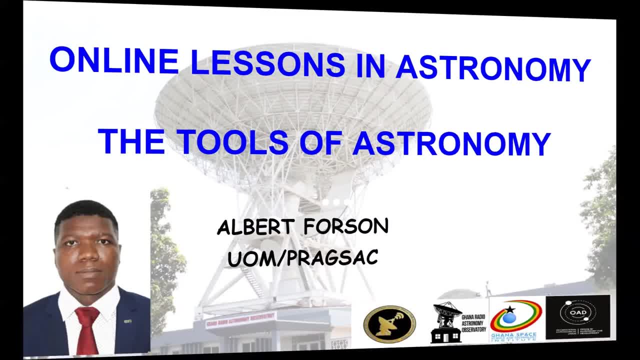 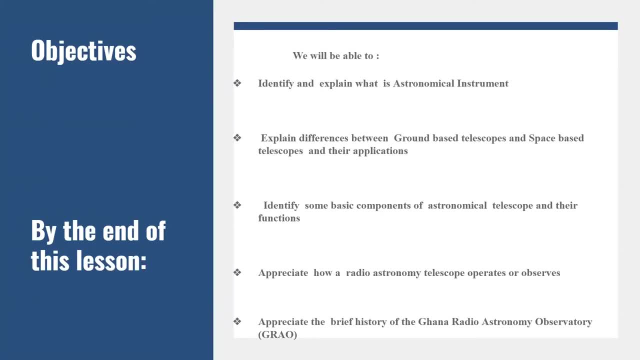 we will be looking at the following areas. So by the end of the lesson, we will be looking at the following areas. So by the end of the lesson, we will be looking at the following areas. So by the end of this lesson, we will be able to identify and explain what is an astronomical instrument. 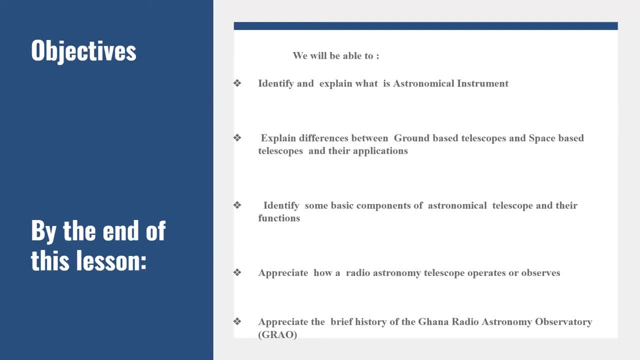 We will also be able to explain the differences between ground-based telescopes and space-based telescopes, and their applications. We will also identify some basic components of astronomical telescopes and their applications. We will also identify some basic components of astronomical telescopes and their applications. We will also find out that Bhayan's overturning got.